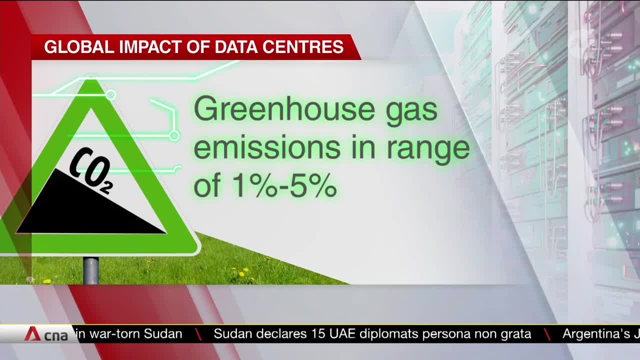 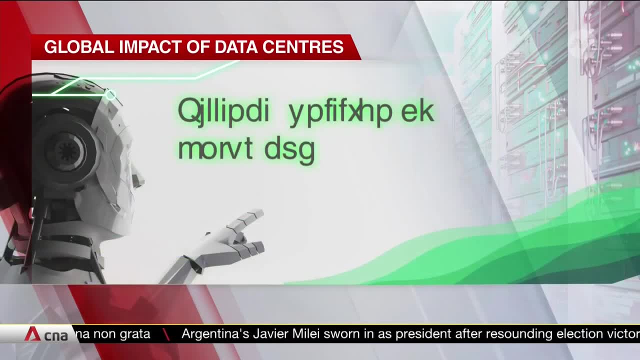 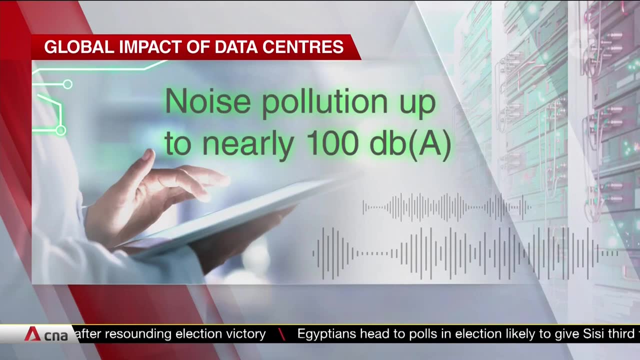 Estimates vary on carbon emissions from more than one percent to up to five percent of the global total, roughly in line with the aviation industry. Data centers also use vast amounts of water for cooling and create noise pollution. The true impact, though, is hard to gauge. 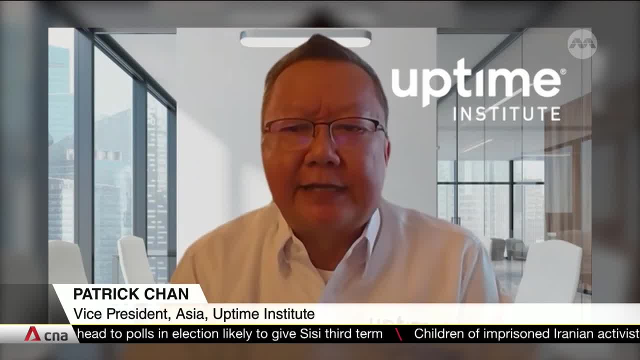 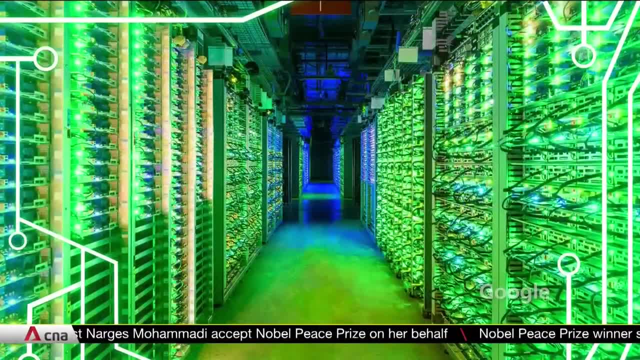 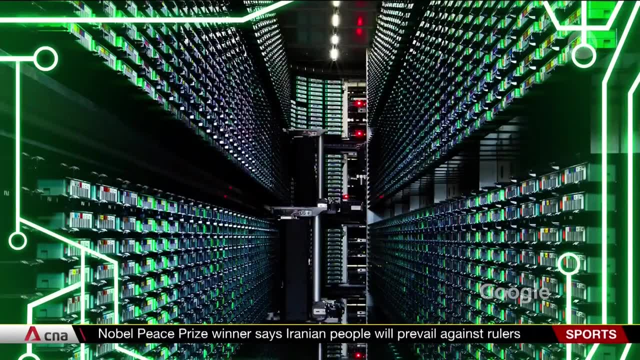 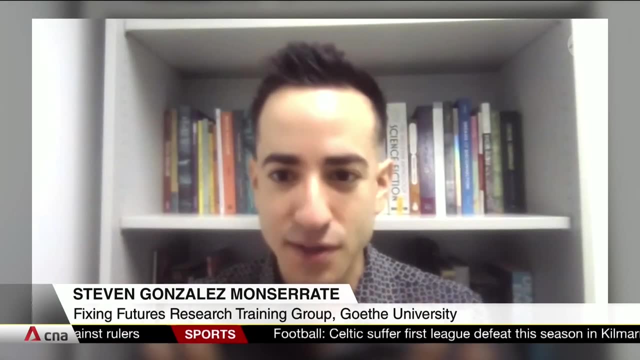 making sure that we're communicating exactly the same fragile values. Most of the database, the data centers in the world- they're not these giants big tech kind of data centers that you see in in many films and so forth. they're actually smaller in scale. they don't have 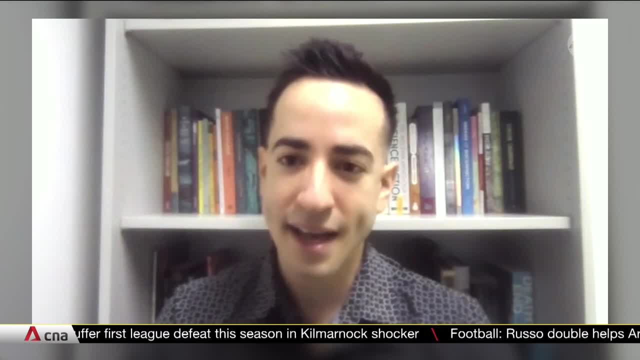 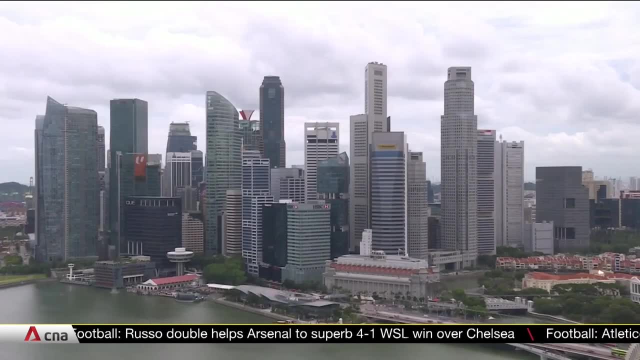 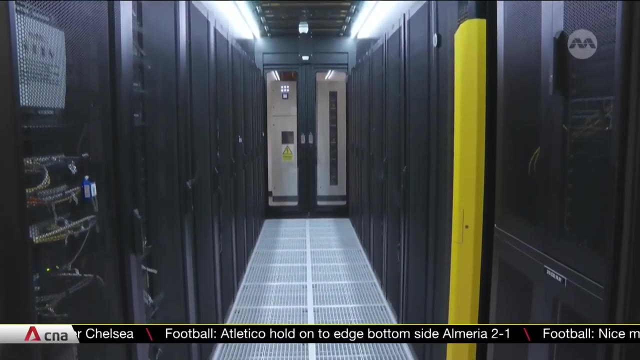 resources. they're not as high tech or sophisticated and, as a result, they also don't have lots of information or insight into their environmental impacts. Hot Tropical Singapore is one nation working to transform data centres. It hosts more than 70 of these facilities and it's being selective about building new ones. 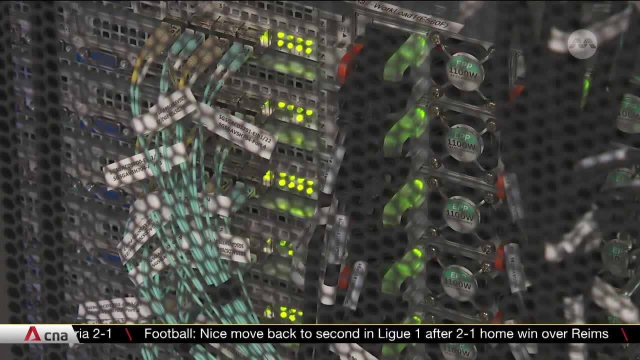 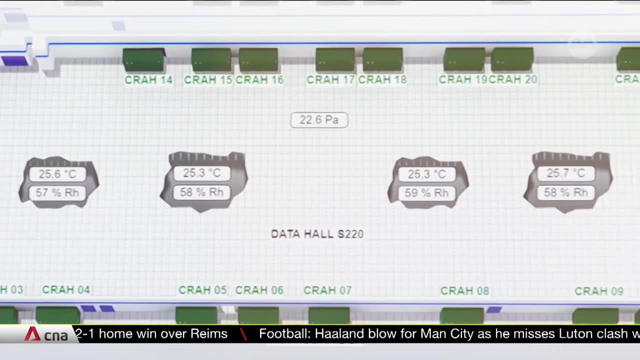 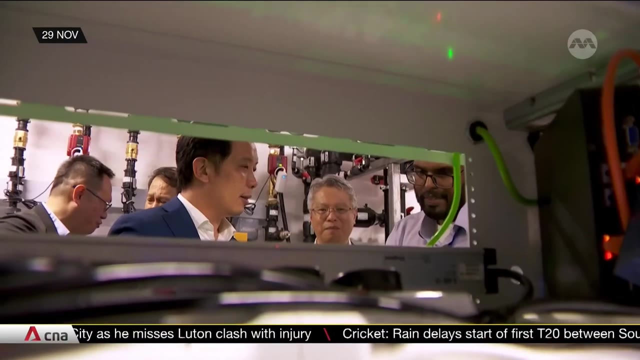 emphasising sustainable growth and low carbon emissions. Authorities set a standard this year as part of efforts to get DC operators to gradually increase temperatures to 26 degrees Celsius and higher, And last month the government unveiled a data centre testbed focused on developing energy-efficient cooling technologies. 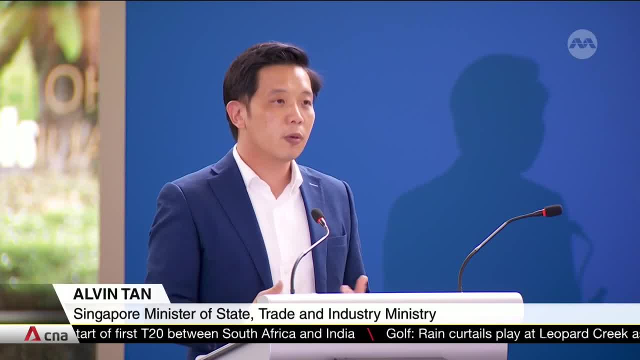 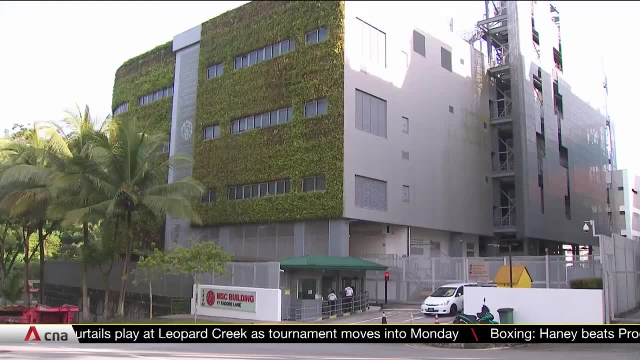 customised for tropical environments. As many of you all know, data centres support our digital economy, and that's critical. We cannot do without them, but we need to make them greener. It's a view shared by companies such as Singapore's Empyrean DC. 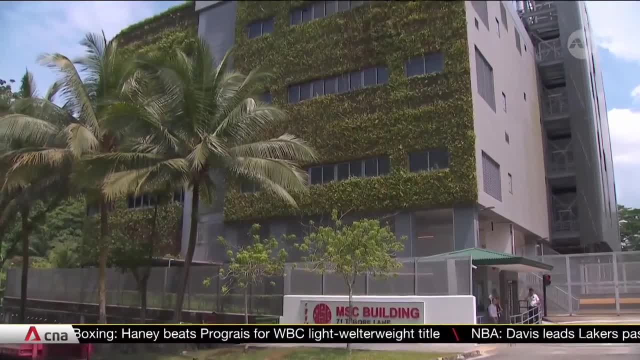 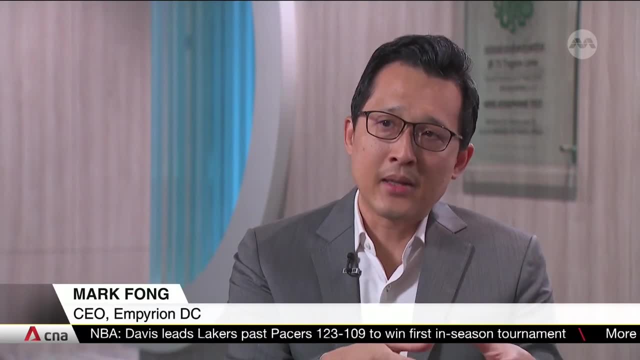 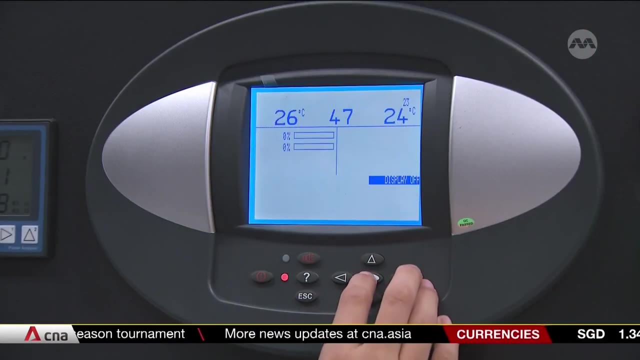 The up-and-coming player has a small portfolio dedicated to being lean and green from the outside in. How do we ensure that we're thinking about it holistically and not just at the rack level or the server? That includes nudging temperatures higher, constantly upgrading technology. 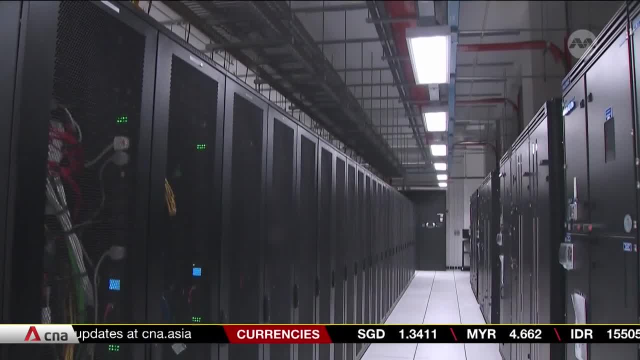 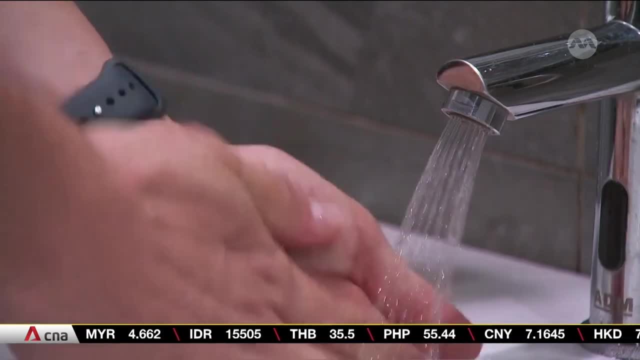 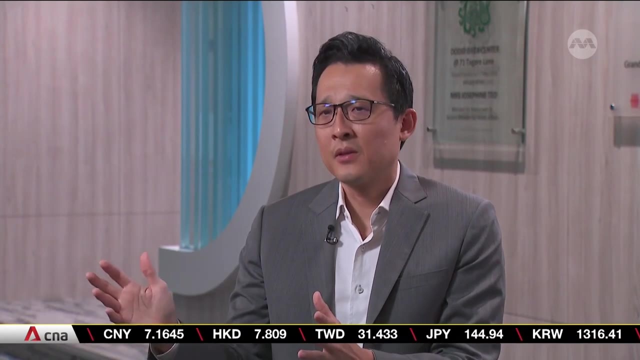 while properly managing e-waste and keeping even the small stuff inside, such as reducing water usage in the bathrooms. The end goal is really to be able to tap off the grid clean energy. 100% would be ideal, unlikely for years to come, but even 50,, even starting, 10,, 20,, 30,, 50%. 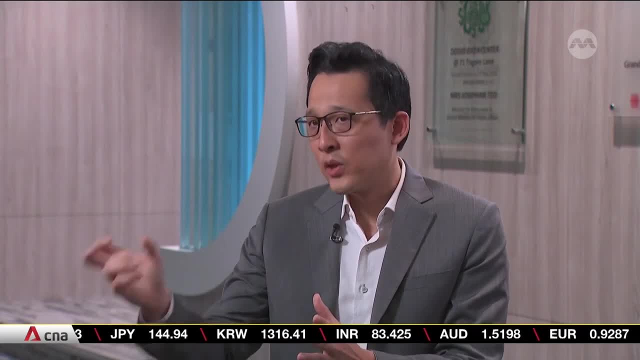 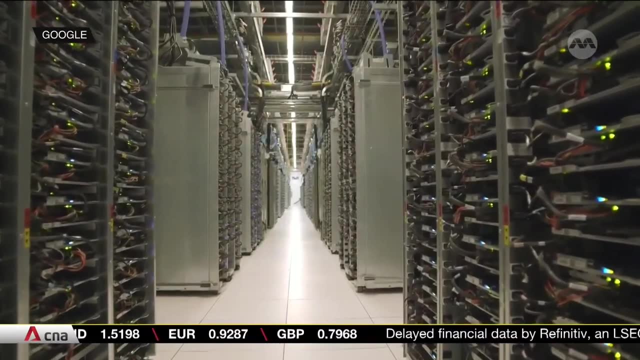 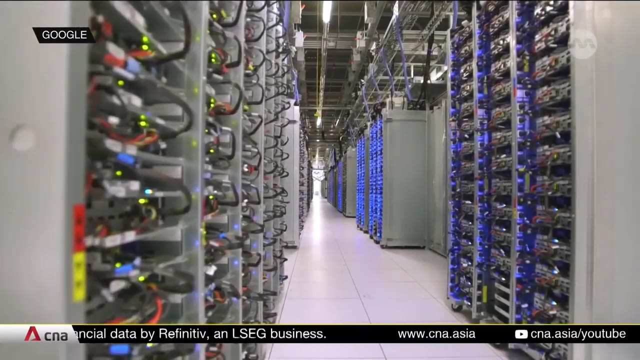 I think that's really where you want to get to, because that's true. What's measurable is also important to the folks at Google. For six years, they've matched 100% of their global annual electricity consumption with purchases of renewable energy- The moonshot for 2030?. 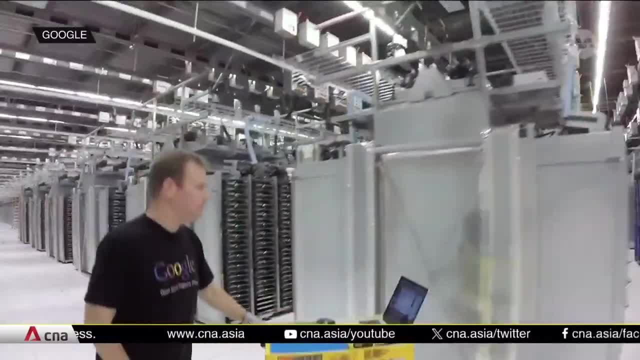 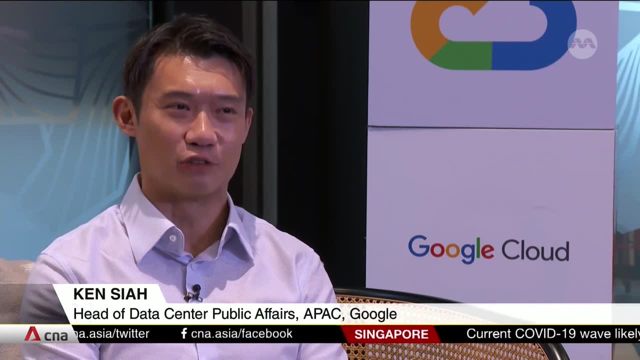 Running on carbon-free energy all day, every day, everywhere. Now, obviously, this is very challenging, right? Like even with the renewable energy, the most advanced renewable energy markets that we have now, the sun is not going to shine 24 hours a day. 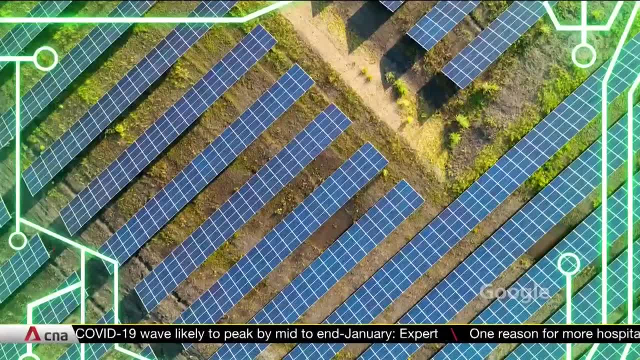 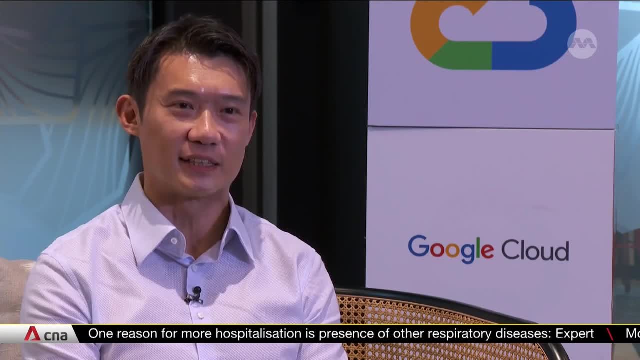 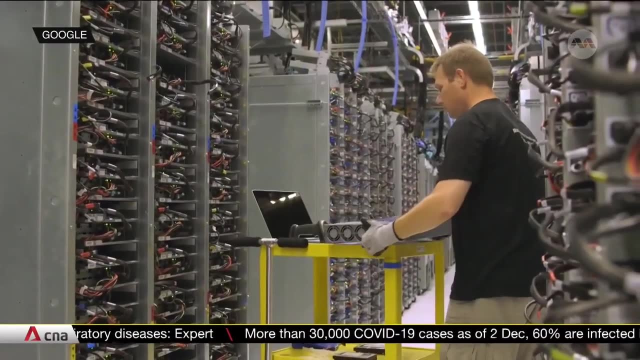 The wind is not going to blow 24 hours a day, So we have to really work with governments, energy producers, renewable energy generators, to make sure that the grid is set up and properly equipped in order to make this transition. This translates to encouraging governments to tweak regulations. 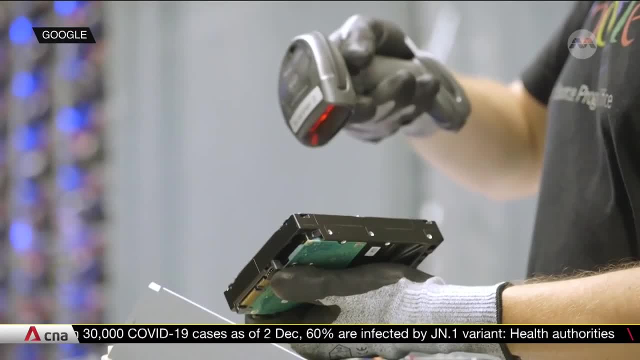 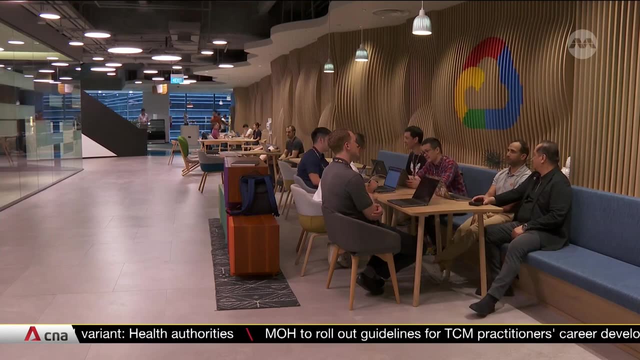 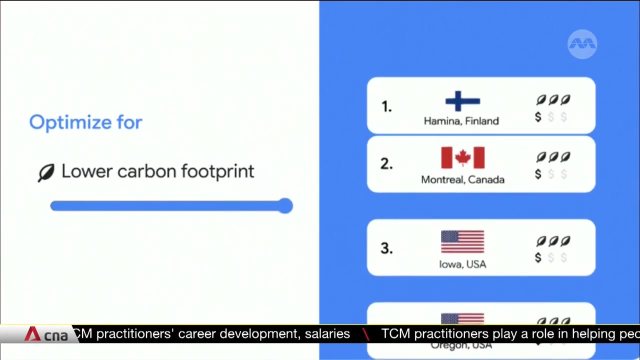 and investing in scores of renewable energy projects globally, but also installing more efficient chips, using machine learning to slash power consumption and thereby emissions, even giving customers a chance to pick where in the world they want to run their cloud computing to meet their own sustainability goals. 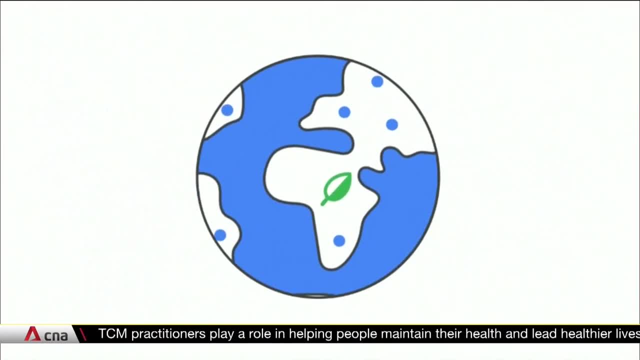 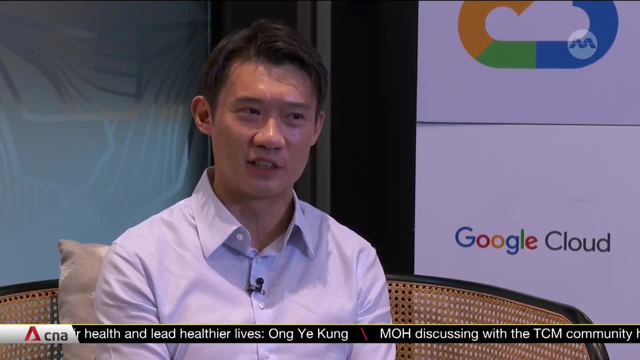 Customers are demanding it, Governments are demanding it. You know it is a business imperative that they have to become more sustainable And I think a lot of companies recognise this And I think that's why, you see, there's a greater push in the industry in general. 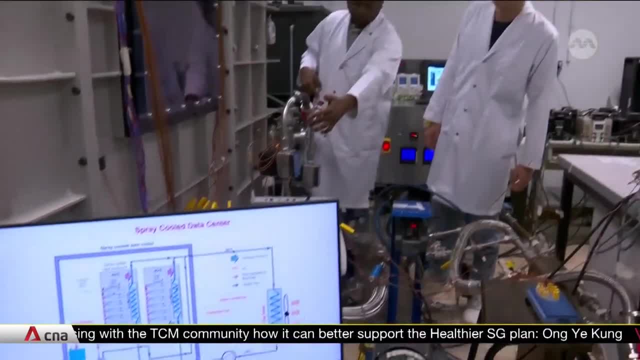 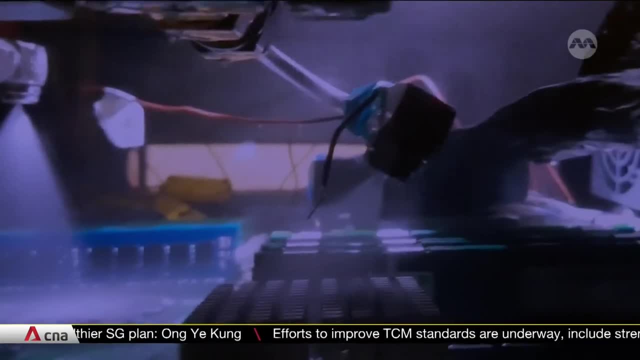 to have more sustainable data centres. Researchers are also part of that push. A team at Nanyang Technological University is using a non-conductive liquid to spray-cool CPUs. So with this invention, there is no chiller-based cooling system required. 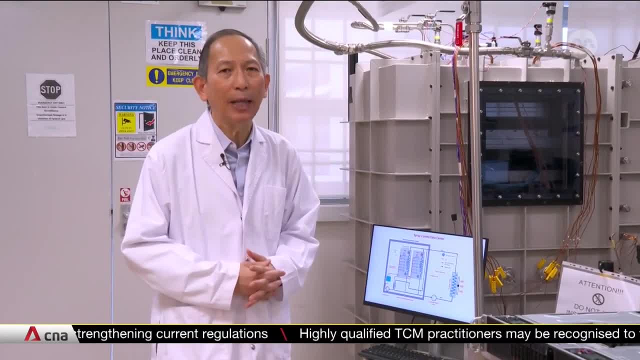 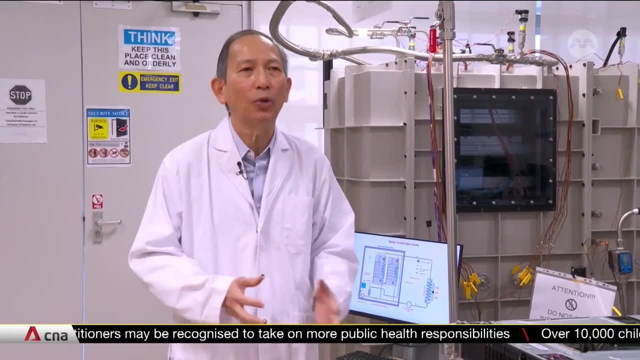 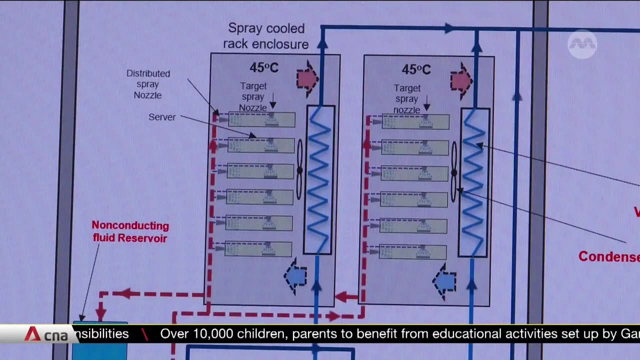 to cool the data centre. The only energy-demanding equipment would be the pump and the fan, So that results in 26% saving in the total energy consumption and also 26% in terms of carbon footprint. Associate Professor Wong Teck Neng says.